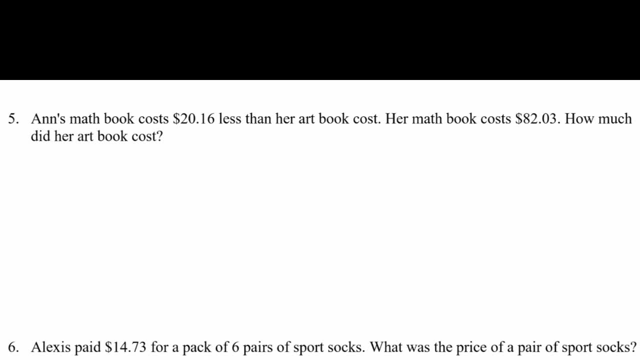 Then her art book cost. Her math book cost $82.03.. How much did her art book cost? So what is the problem asking us to find? It says: this last sentence kind of gives us a big clue. It says: how much did her art book cost? So that's our unknown quantity. So we're going to name that quantity. Shall we call it X? How about if we use X And we're going to have a declaration statement that says: 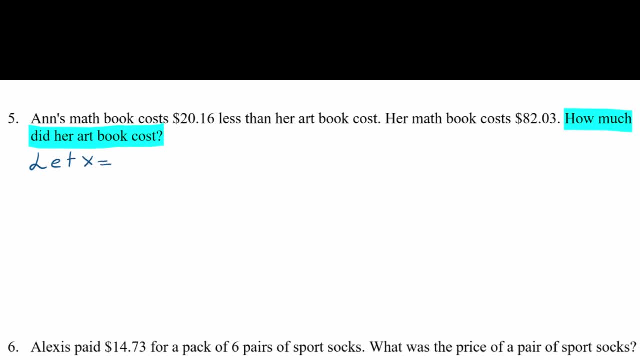 We're going to make very detailed. So what are we asked to find? We're asked to find the cost of the art book. It says how much did her art book cost. So we're going to let X be the cost of her art book. 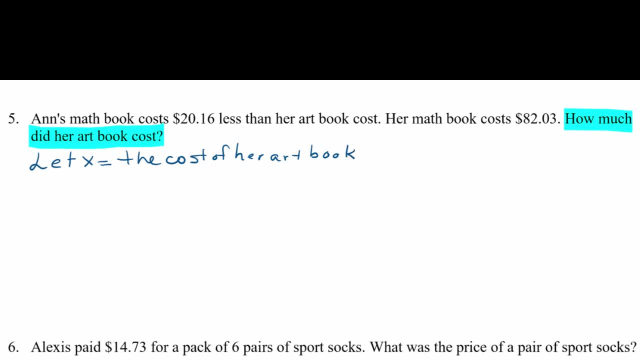 Okay, one thing I want you to notice is that I did not write X equals art book. That would give me no information whatsoever if I say X equals art book, because I wouldn't know. Is it the size of the art book? Is it the number of art books that I bought? Is it the cost? I mean, it's not enough detail, right? So make sure that when you set up this declaration statement, you are very precise, And let me tell you that your math teacher will be so impressed. I'm going to tell you from experience. Okay, so let X equal the cost of her art book. 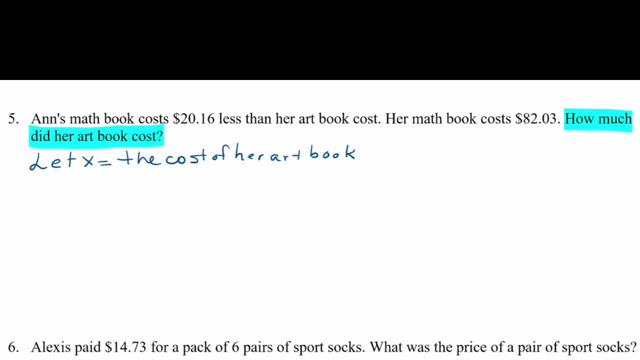 What else is given in the problem? Well, we know a couple of things. We know that the math book cost $82.03.. So we're going to use that. But it says here that that math book cost twenty dollars sixteen cents less than the art book cost. let's. 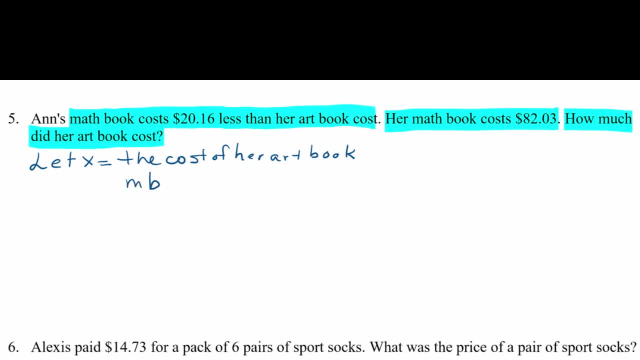 think about that. so math book, math book costs 2016. less than we talked about, less than in the last video: the art book, art book cost. what are we letting the art book cost represent? what? what are we using for that unknown quantity? if you said X, you're right. so this is our X, isn't it? and then we know what to do. 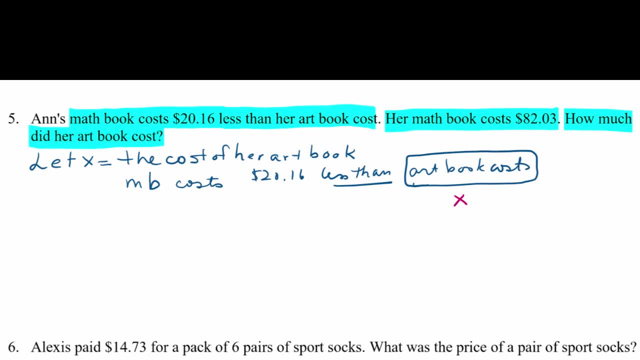 with less than we know that this 2016 is going to go behind the subtraction symbol. we talked about that in the last video, so it seems like over here we have X subtract the 2016. what do you think? twenty dollars sixty cents less than the. 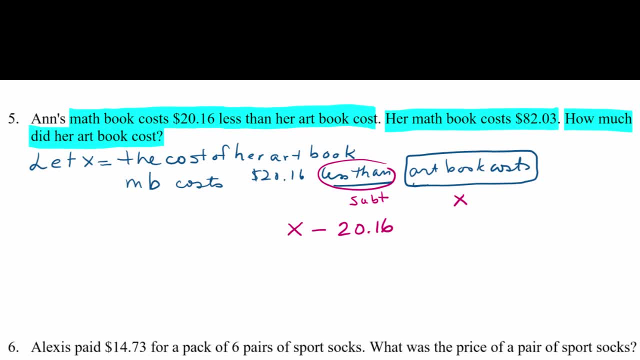 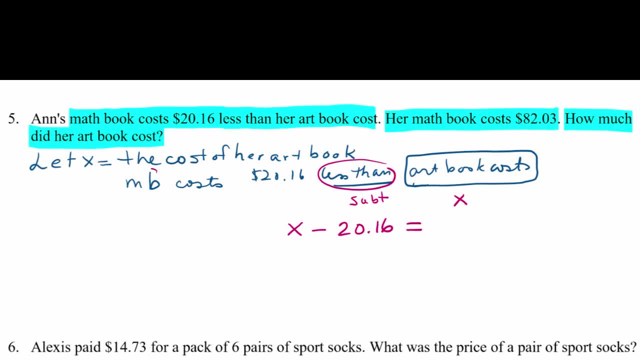 that equals. and what do we know about this math book cost? we know it's $82.03, so that equals $82.03. so there's our equation, using the given right, the key words in the problem, and now we're gonna solve for X. this is linear equation: X to 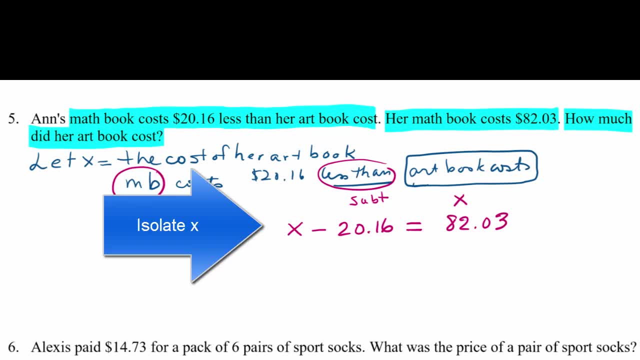 the first. so we know we need to isolate X, which means that we're going to have to add 2016 sides of the equation right so that we can get this X by itself, and so X equals. what is that? let's see: a hundred and two dollars and 19 cents $102 minus 2016 is. 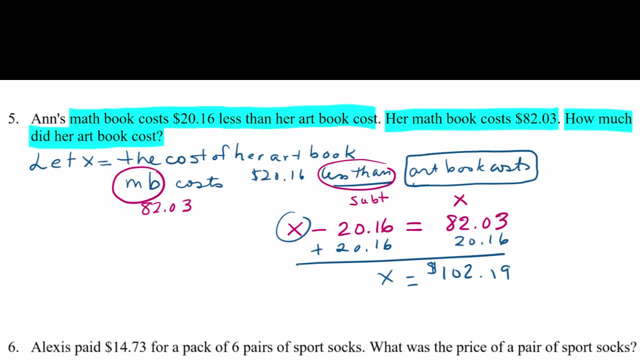 82, oh three, that makes sense. so it makes sense that the art book costs more than the math book, doesn't it? that's one of the things you want to think of. well, yeah, because it says that the math book is less than her art book. right, so that? 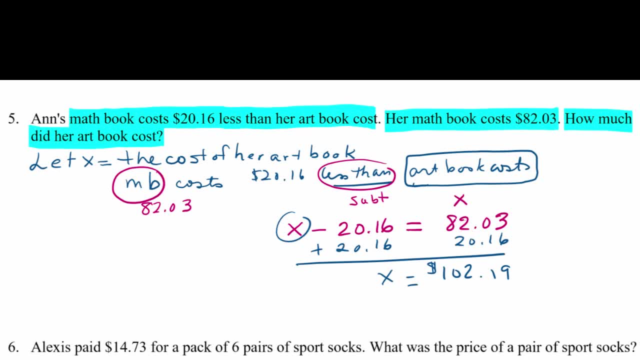 makes sense. so let's answer the question. and- and you want a complete sentence, ah, so impressive. when you do that and our book costs a hundred and two dollars and 19 cents, well done, okay, we're gonna go to number six here. we have Alexis paid $14. 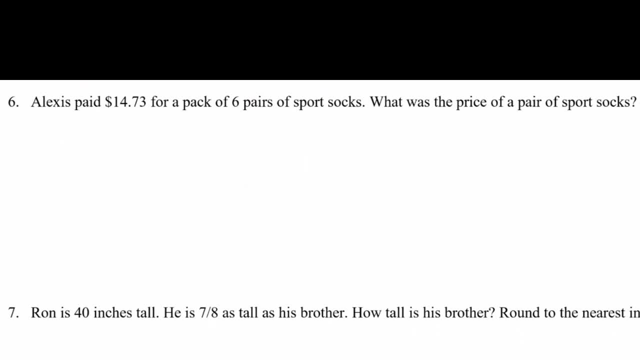 and 73 cents for a pack of six pairs of sports socks. what was the price of a pair of sports socks? so, one pair of sports socks, okay. so what are we asked to find? the price of a pair of sports socks, that's what we're asked to find, right, so that's. 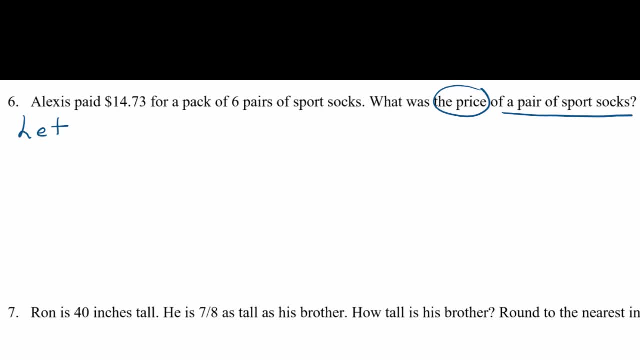 going to be our unknown quantity. we're gonna choose a variable. we're doing this via algebra. you're probably liking. it's going: oh, I can do that in my head. I can do that. I don't need an algebra equation, but it's gonna. goodbye, that's all. we're gonna move onto number nine. 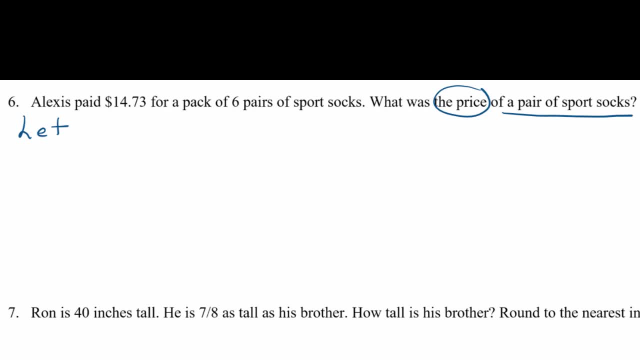 four, we're going to move on math. so, like we said, there's a few questions we have. but that's not false, but I. But if it's part of your homework and your instructor is asking for an algebra equation, you've got to give it to them. 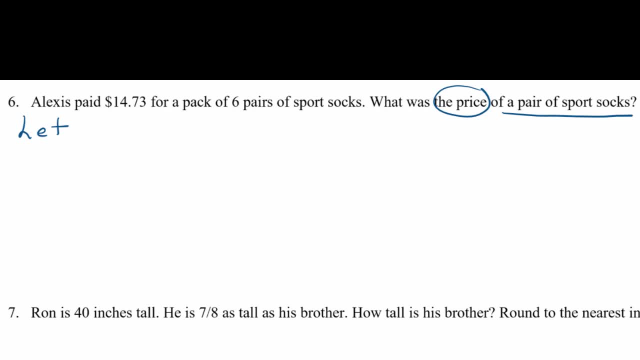 OK, so. so let's set it up. It'll be good practice. for a price of a pair of sports socks, Shall we use S for sock, Let X be the price. OK, notice again what I did not do. I did not write. S is a sock. 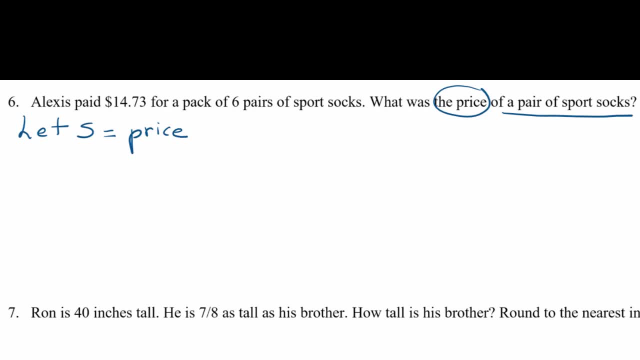 No, I wrote: X is the price of a pair of sports socks, because that's what we were asked to find. So that's, you're going to declare your variable with a lot of detail. And then what do we know about this? S Well, that a pack of six of those is fourteen dollars and seventy three cents. 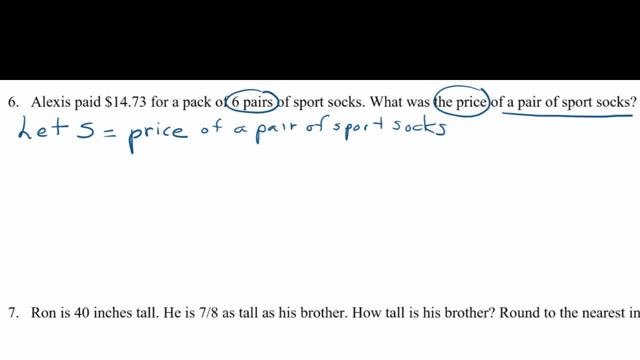 A pack of six pairs. So that means multiplication, doesn't it? Six S. So multiply six pairs times The price of one pair of socks. that gives us the price for the whole pack, which we know is fourteen dollars seventy three cents. 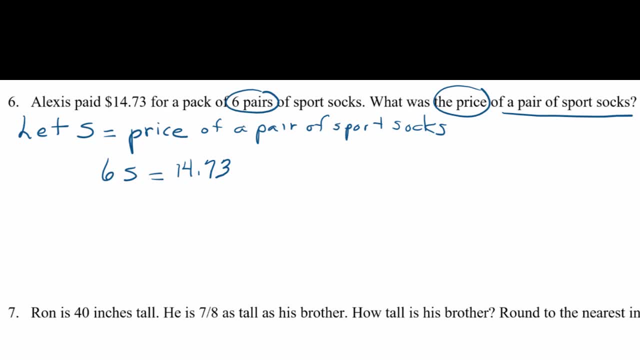 So there is our algebraic equation. Not a bad one, right? And to solve it, to isolate it, S we're going to divide by six, which we knew we were going to do, right, You were probably. you're like I knew. I knew that's what I was going to do, without doing all this algebra. 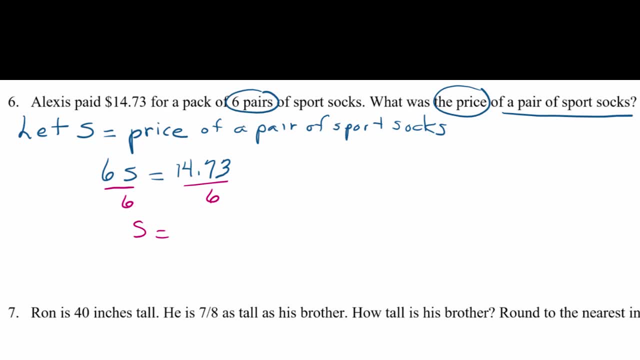 But again, it's good for us to have this practice. OK, let's do this division. So I took this to my calculator and it It says: here's the answer that it gave me. The calculator gave me two point four, five, five right. 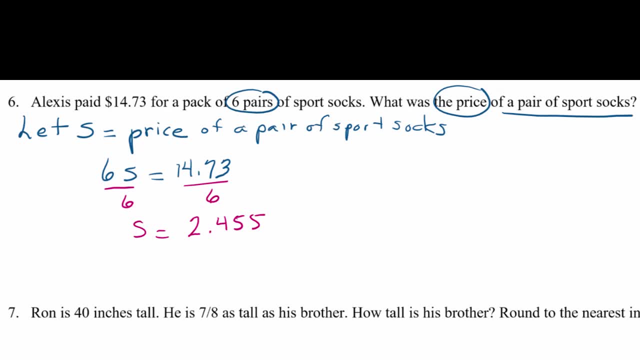 OK, but what did we just find? What did the problem ask us to find? It asks us to find the price of a pair of sports socks. I don't know about you, but I haven't had half of a cent right. 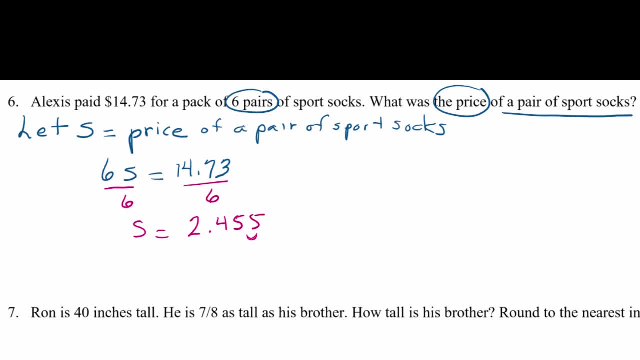 There's no such coin. So we're going to have to do some estimation, We're going to have to round this And we will. So we use the property where we round up because of this digit being a five. so we should round that up to two dollars and forty six cents. 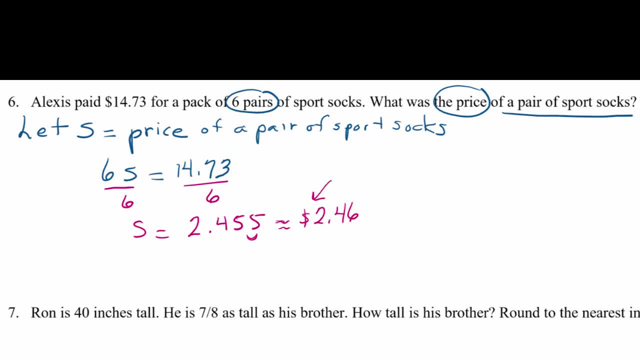 The units are very important. So, and when we multiply, when we multiply this answer times six, we get a little bit more than the 1473 because of the rounding Right. But let's answer the question. So the question is: the price of a pair of sports socks is two dollars and forty six cents. 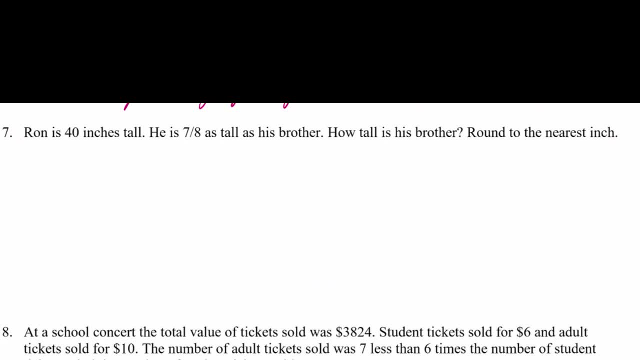 Make sure you write all your units and be very clear. In number seven we have, Ron is 40 inches tall. He is seven eighths as tall as his brother. Oh, that's interesting: Seven eighths as tall as his brother. 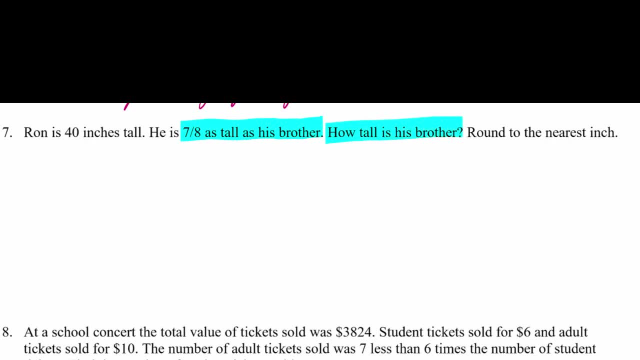 How tall is the brother? How tall is the brother Round to the nearest inch? Oh, they wanted in inches. So this is important. We got some good information. What are we asked to find? Did you say height? You're right. 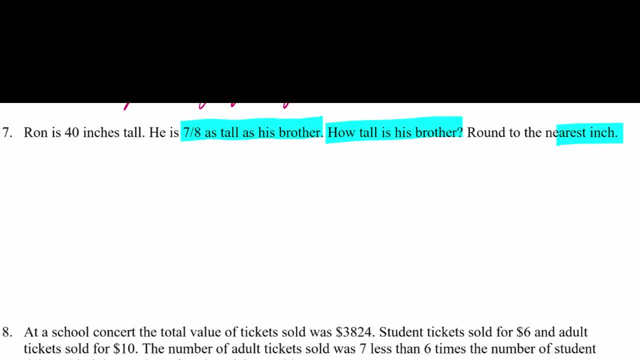 Whose height? Do you think it's eight? Do you think brothers? Ron's brother, You're absolutely right. Let X- Should we call it H- for height? Yeah, let's do that. Let H be the height in inches of Ron's brother. 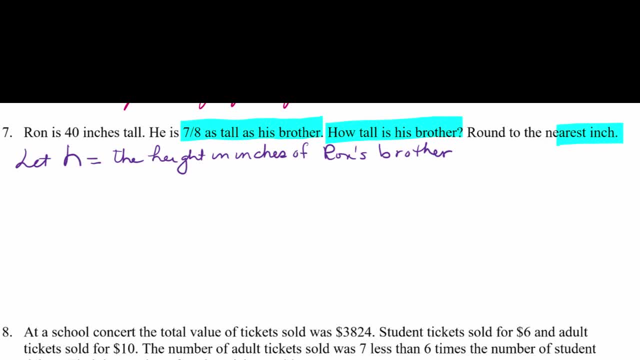 Notice all the detail. Please don't write H equals height or H equal brother or B equals brother, because that doesn't give us enough detail. OK, so Ron is 40 inches tall, so he is seven eighths as tall To be as tall as his brother. his brother, this height, we've decided this is going to be our H. 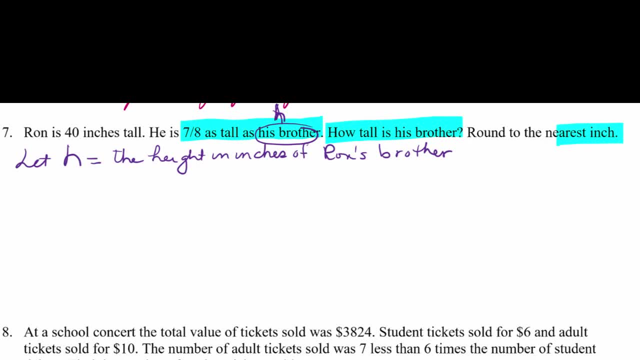 So the brother's height is H, Seven eighths as tall. the way that you do that computation is a multiplication. So seven eighths as tall as H. we're going to write seven eighths H. OK, it is a multiplication to do. 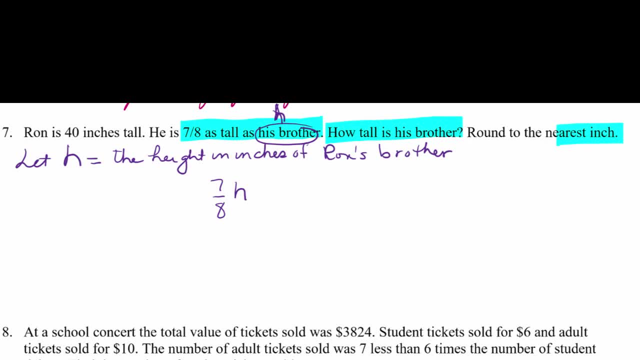 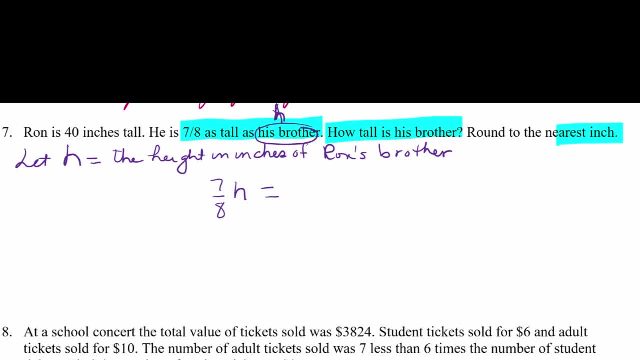 OK, OK, OK, OK, And that is Ron's height. but we know Ron's height That was given to us. That is 40 inches. So we're going to set up this equation with 40 as the height for Ron. 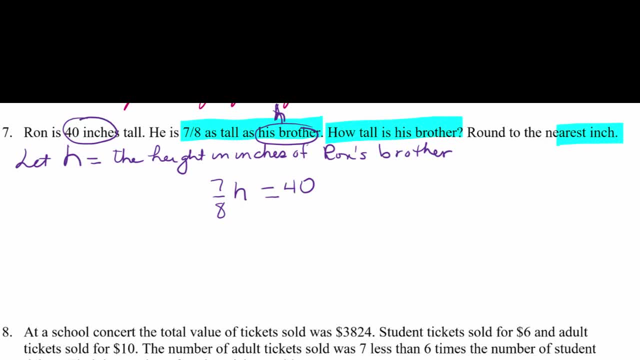 And now again we've got to isolate that H. This time we have a coefficient that's a fraction, This seven eighths, that's a coefficient, that's a fraction. So we know from previous work that, in order to isolate the H, we can use the reciprocal of seven eighths. 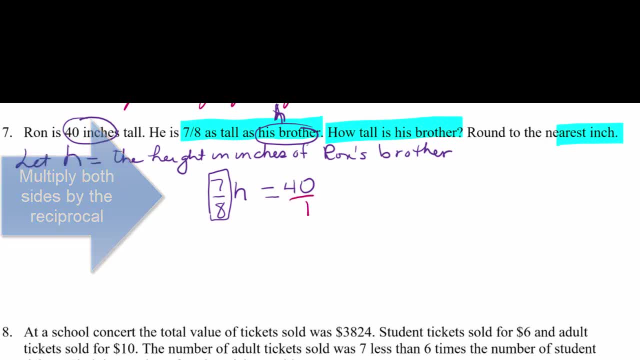 OK, OK, both sides. so I'm going to put a 1 under this 40, and then I'm going to use the reciprocal here and go times 8 sevenths, and then I'm going to use times 8 sevenths here and again. why did we do that? because now these eights give us ones. 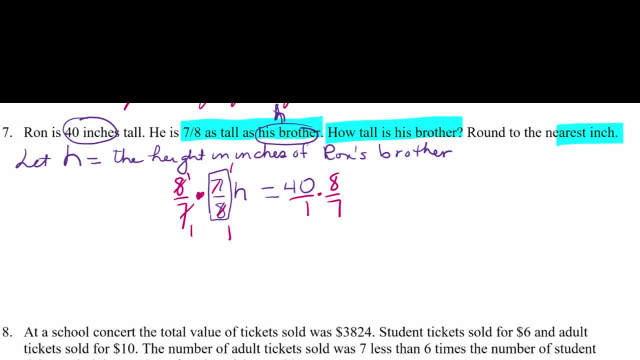 and these sevens give us one. so we have one H on the left, which was our goal. okay, over here on the right hand side, we're going to go ahead and multiply straight across 320 over 7, and then we've been asked to round that to the. 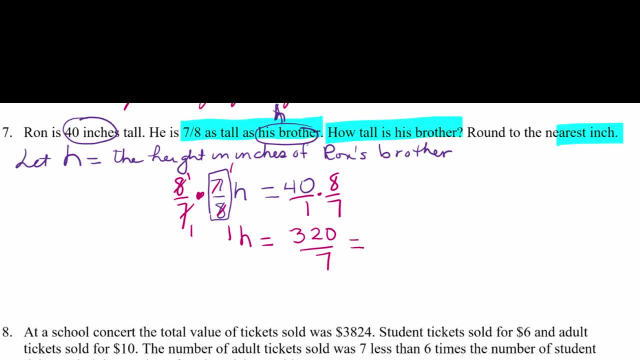 nearest inch. so it is appropriate for us to go to the calculator and figure out what this division is. I'm getting 45.71, etc. right, but they want nearest inch and that would be the 5. that means we want to round to this place, right? the 7 tells: 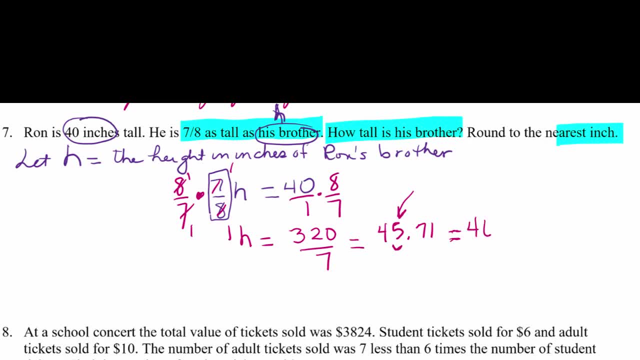 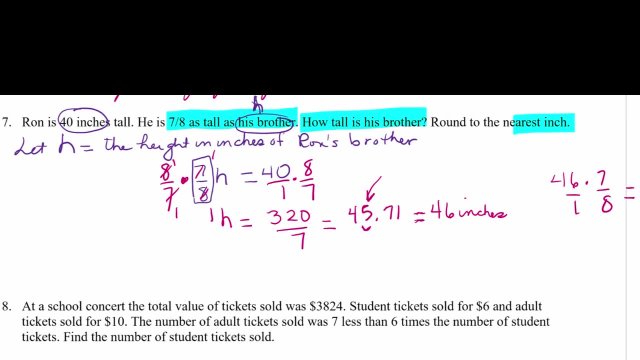 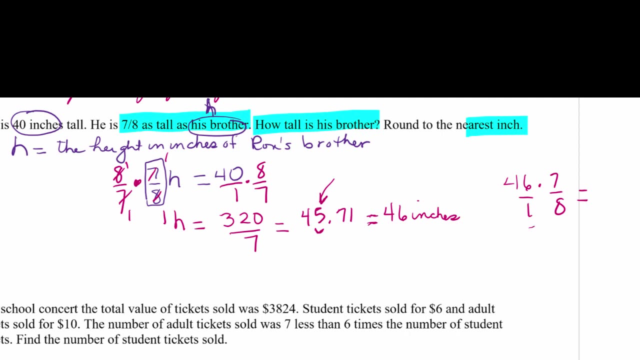 us to round up to about 46 inches. and if we do a quick multiplication in the calculator, times 7, eighths, right, if you do that in your calculator, 46 times 7 go straight across. that's 322, and 322 divided by 8 is 40.25, so it's. 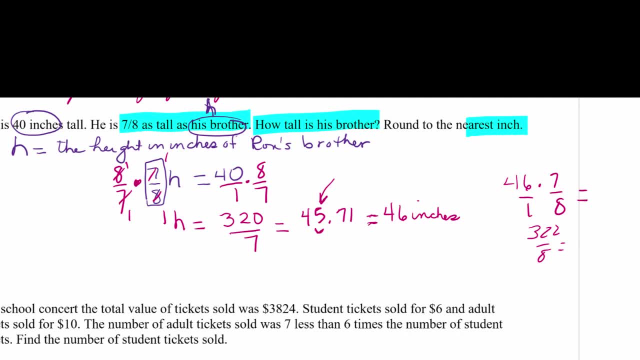 about. it's around the 40 inches. right, it's a little bit more when we check because we approximated, we round it. so that's good, that's a good check. oops, 40.25. that's a good check. so now let's answer the question, Ron's. 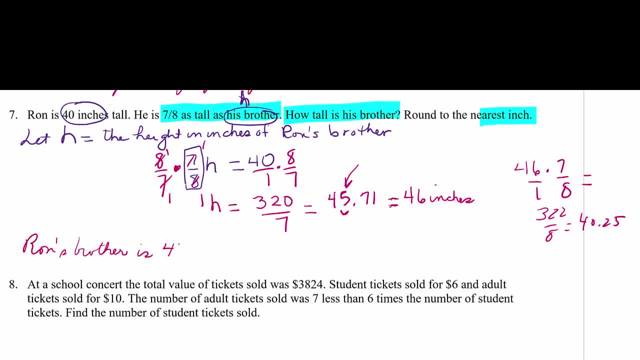 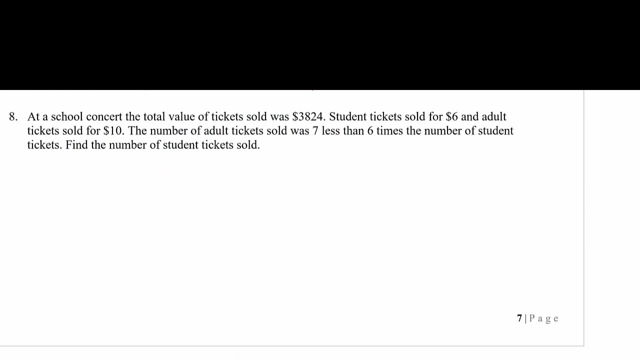 brother is 46 inches tall, or you can write approximately 46 inches tall, but that answers the question: how tall is the brother? problem 8 says at a school concert. the total value of tickets sold was 3 thousand eight hundred and twenty four dollars. the student tickets sold for 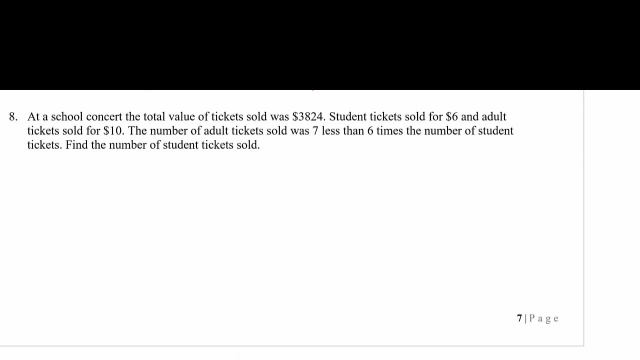 six dollars each and the adult tickets sold for ten dollars. each one is a six dollars and another beat is six dollars, but that знт is 32 dollars, which makes 36 total values. in the story, the number of adult tickets sold was seven less than. oh, there's our less than. 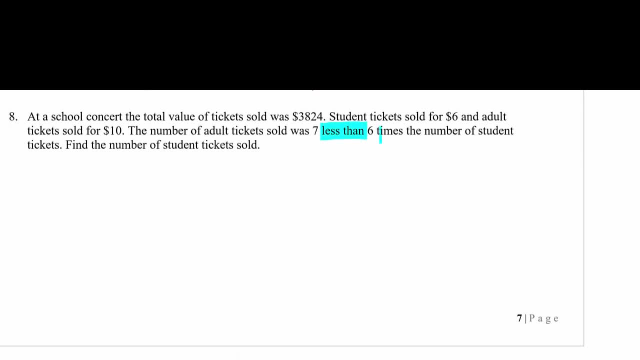 seven less than six times, six times the number of student tickets. find the number of student tickets sold. so what is the problem asking us to find? it's asking us to find how many student tickets were sold. so I'm going to use s for student student tickets and I'm going to write: let s s be the number of. 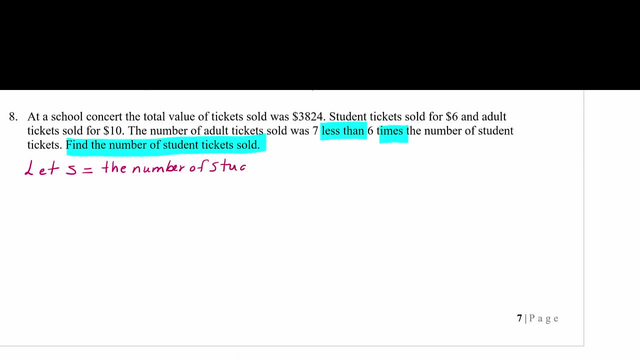 student ticket sold. you see how that last sentence really helps to kind of tell me what to let my variable represent. so let s be the number of student tickets sold. so when we read carefully the given problem, we can tell what our variable should represent. it says we now need an expression for the number of. 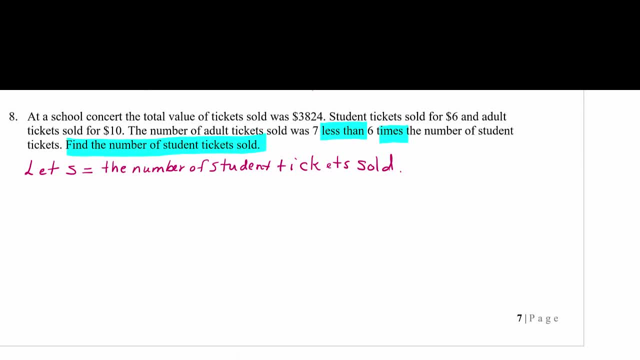 adult tickets sold. because this problem, do you notice? we have a lot of information. we have information about the total value of tickets sold. we know how much the student tickets sell individually and the adult tickets, and we know something about the number of tickets. do we know? so we're going to 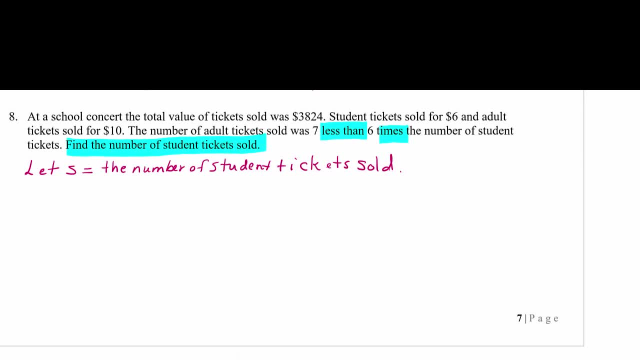 need to represent the adult tickets as an expression based on the number of student tickets sold, and so we're going to use this sentence right here. that's next to the last one. so s is the number of student tickets sold, and then the number of adult tickets sold is seven, less than six times the number of 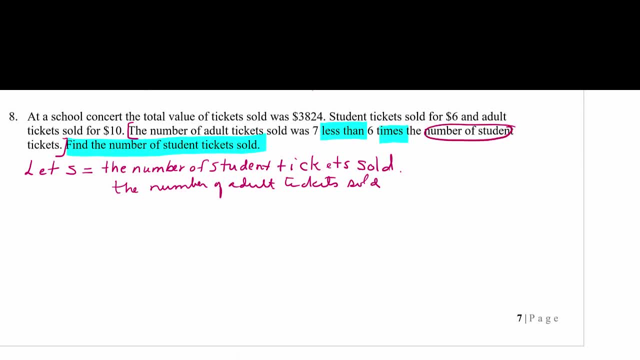 student tickets and the number of student tickets. we have used an s to represent that and we have need six, six times that. so six s and. but if there's seven less than, remember less than, we put the seven after the subtraction sign. so six s minus seven is an algebraic expression that represents how many. 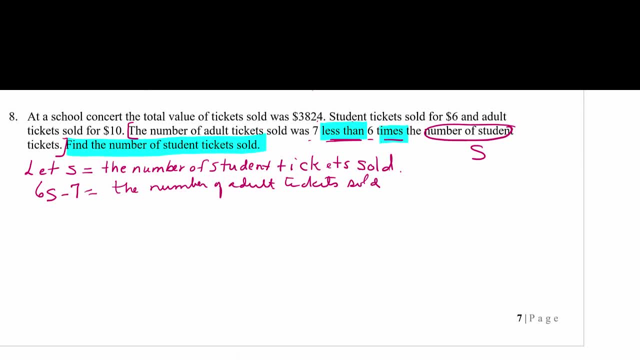 adult tickets were sold. why do all that work so that we can find this s right? so what information haven't we used? well, we haven't used these first two sentences. our equation is going to have to do with the total value of tickets that were sold, this 3824. and now how do we compute a total value of? 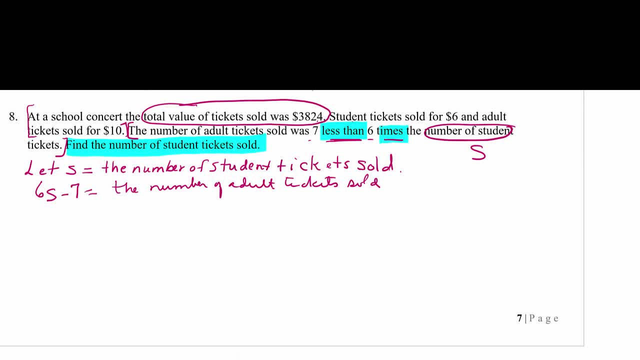 tickets. how do we normally do that? we know that the student tickets sell for six dollars. if we knew we sold five tickets, five student tickets, we would know that we collected $30 for the student tickets. right, and how do we figure that out? because we multiply the six dollars each times the five, which is 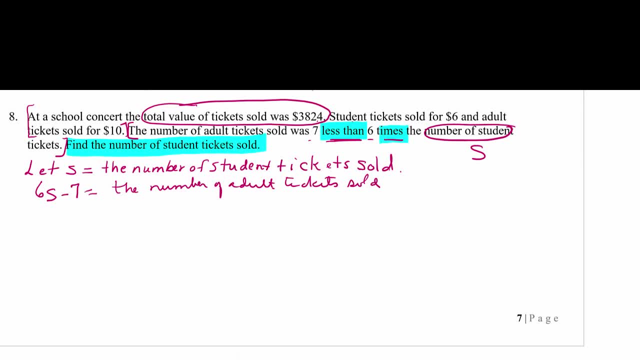 the number of student tickets, right? so when we multiply the six times the five, we get the total cost in student tickets, right? and if adult tickets? adult tickets are ten dollars. so let's say we sold nine adult tickets. so then how much money did we collect? nine times ten, ninety dollars, right? so to figure out. 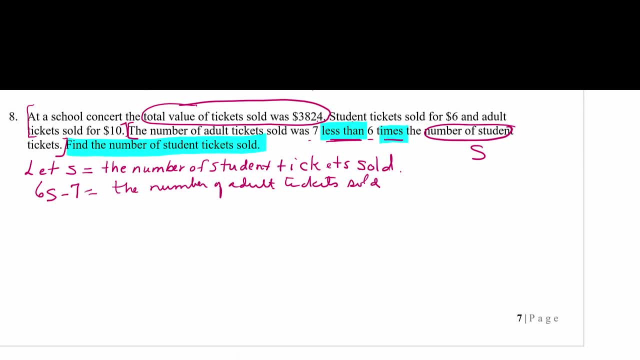 the value. to make an equation, we know we're gonna have to multiply- and what each student ticket sold for. so the ticket value times the number of tickets sold. that will give us the value of the tickets, the total value, so the money collected right at the box office. and so I'm just 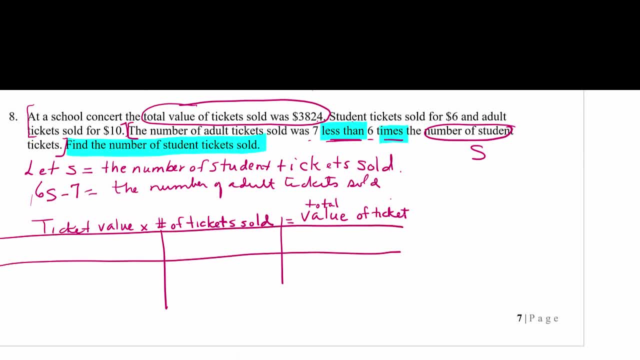 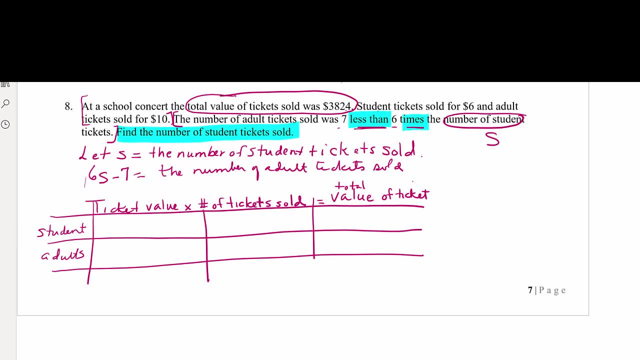 making this little, if this helps you to kind of understand this little table. so we have student student tickets and we have adults. this is done at X. this is at times times okay. this ticket value of student tickets is six dollars each and the adult tickets are worth ten dollars. and how many student tickets that we? 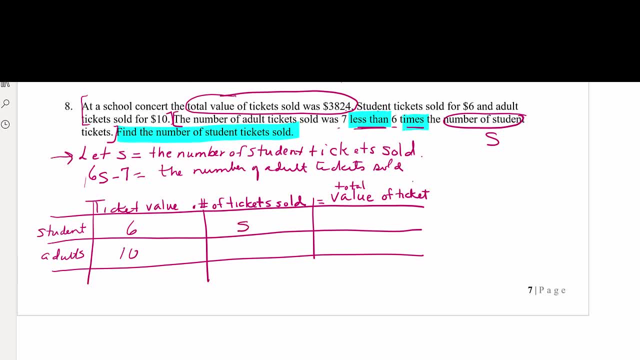 sell? we sold s of them. right comes from here. and how many adult tickets did we sell? we sold six s minus seven. so how do we figure out how an expression for the amount of money collected from student tickets we multiplied six times s, or six s, and in? 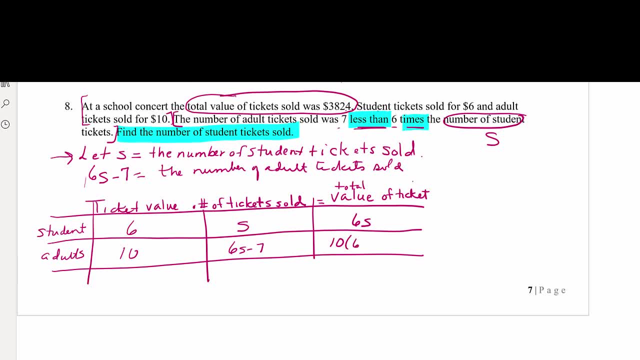 adults. we're gonna multiply here as well, but we are gonna need a parentheses this time. and then, what do we know about 6s? when you add it to ten times six s minus seven, how much total money was collected? thirty-eight twenty-four, so thirty eight twenty four is the total value.